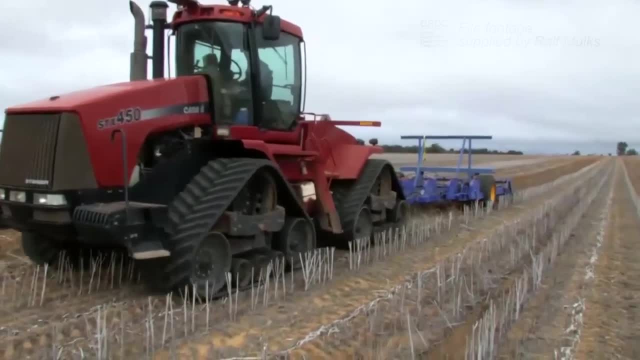 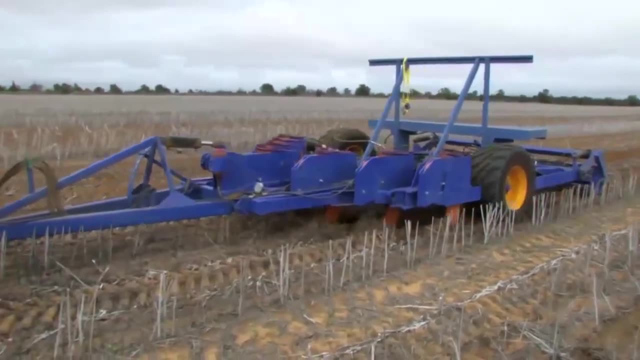 we may see them still performing reasonably well. Paul says that topsoil slotting is a simple way to get topsoil into the subsoil with a deep ripper and could potentially improve plant root penetration where compaction, acidity or sodicity are a problem. 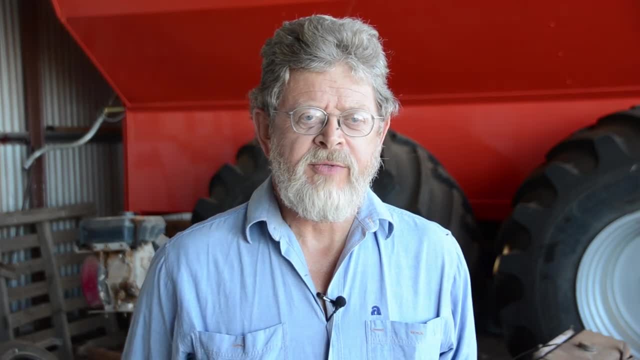 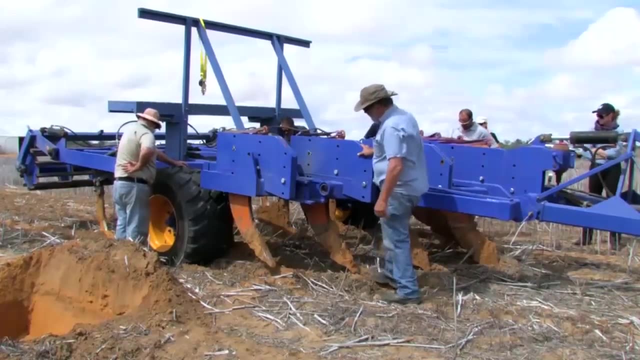 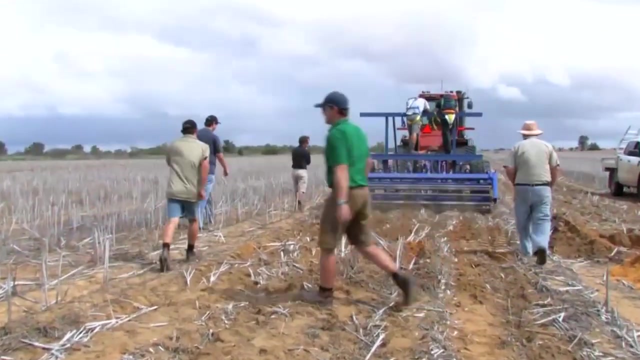 The most commonly available organic matter on the farms is actually the topsoil itself. So the idea of these plates is to get more of that material into the subsoil. We saw something of that effect with some cargo funded trials run by West Midlands Group. 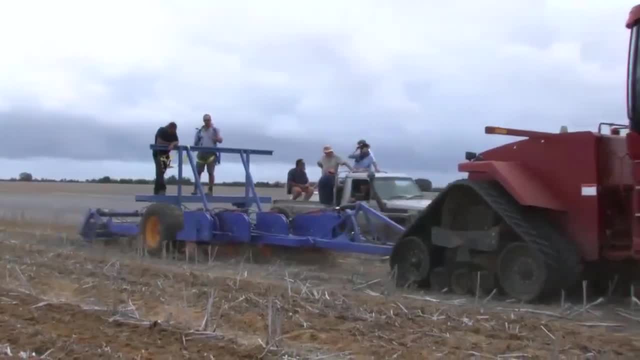 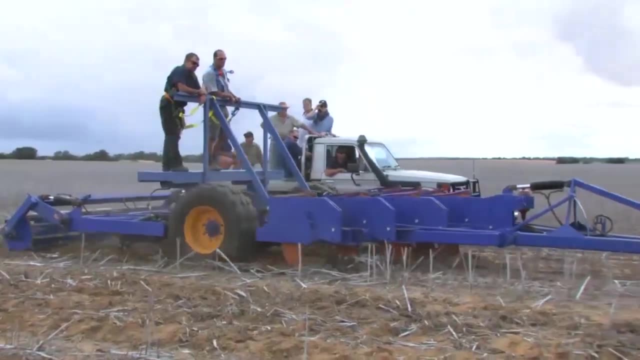 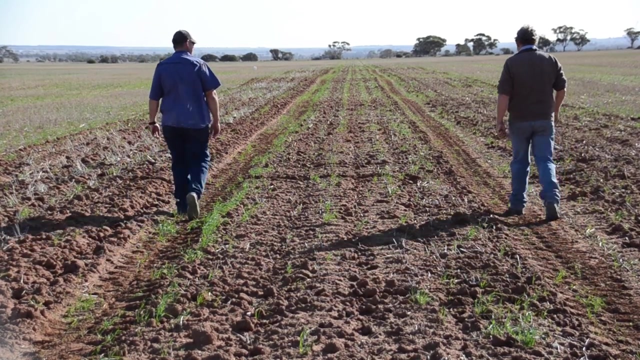 last year or the year before, where they attached, behind times, quite small pieces of metal and the topsoil fell quite readily down behind them. Subsoil farmer Stuart Faulkner is hosting a trial site and hopes to get a better understanding of the full cost of subsoil constraints. 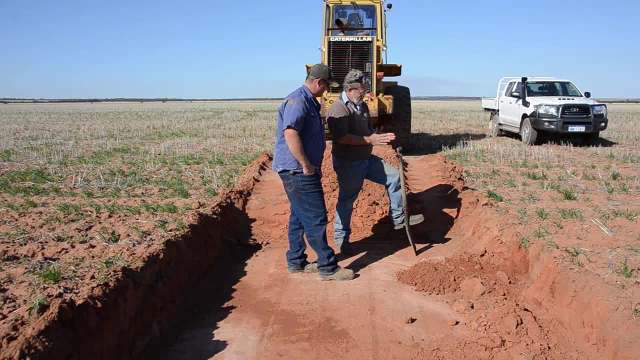 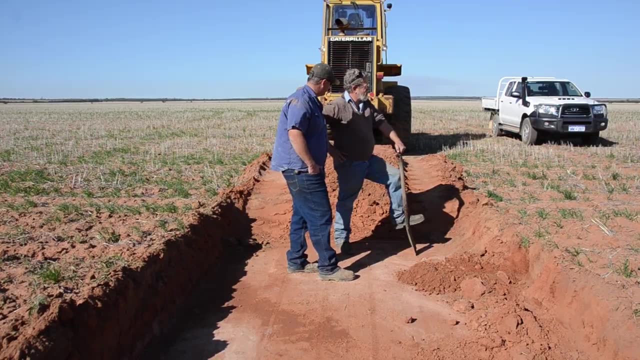 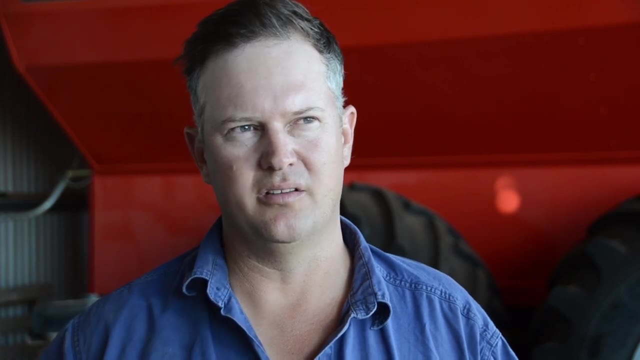 He and brothers Raymond and Jason, started controlled traffic farming in 2009 after realising that compaction issues were costing them grain yield, and it's paying off. We're finding lower draft with the seeders. the soil is much more friable. the seeding- 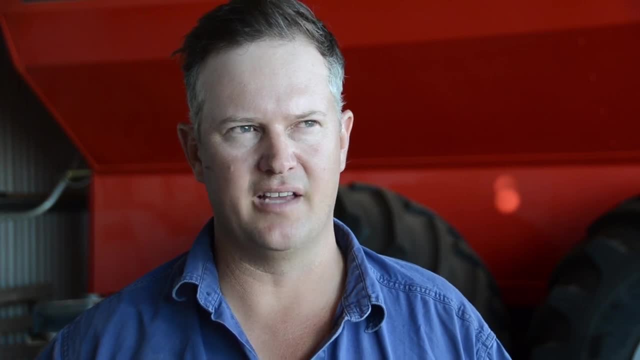 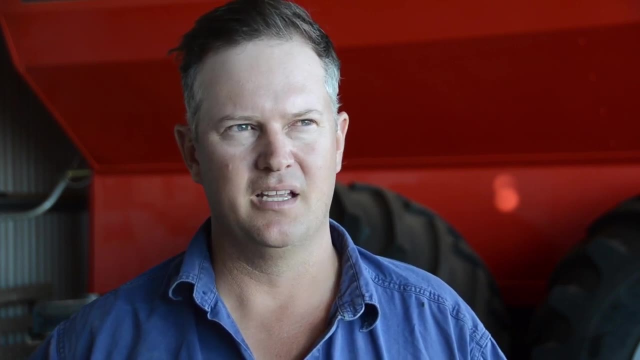 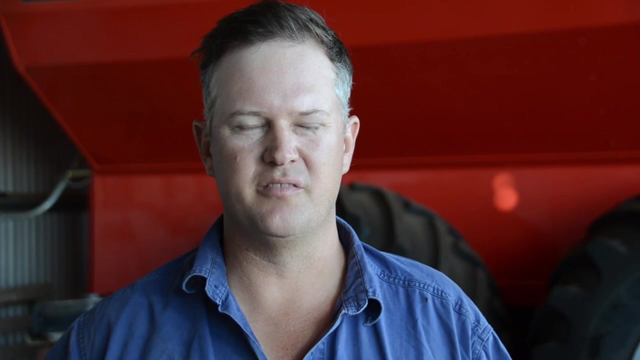 machines are running on a hard traffic track, So they're not slipping or anything. they're getting very good power to the ground, good fuel efficiency usage. As for spraying, one that we hadn't really thought would become a positive, but by having 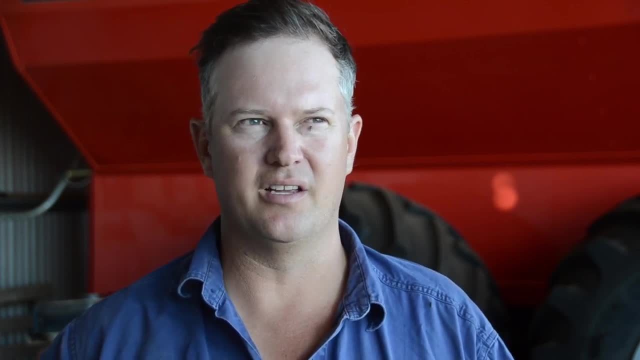 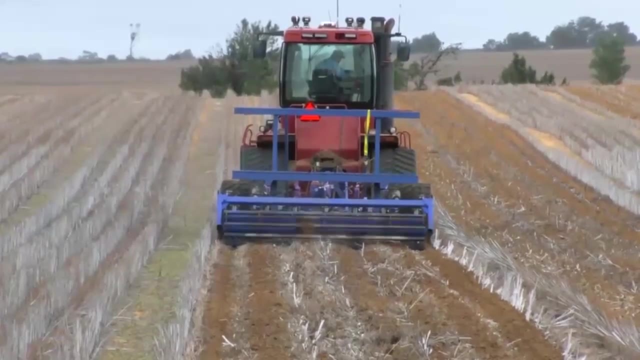 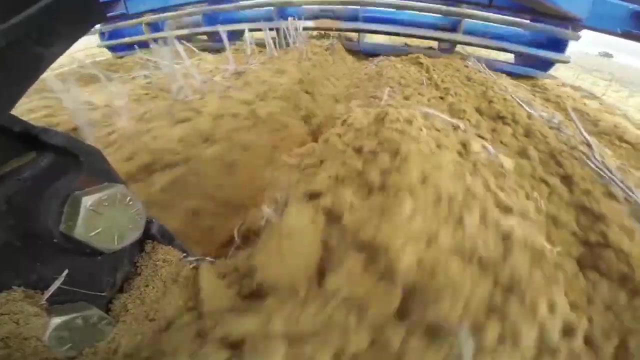 that nice hard traffic road. we're not having so much dust issues when we're summer spraying and things like that. Stuart says he's particularly interested to see how the stabilising techniques will enhance the deep ripping and controlled traffic operations. With our controlled traffic, deep ripping and then hopefully getting some gypsum or the 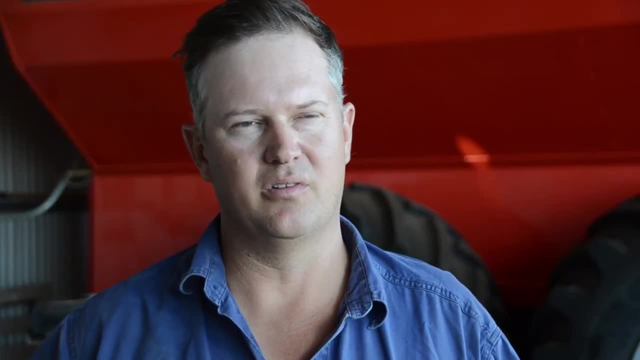 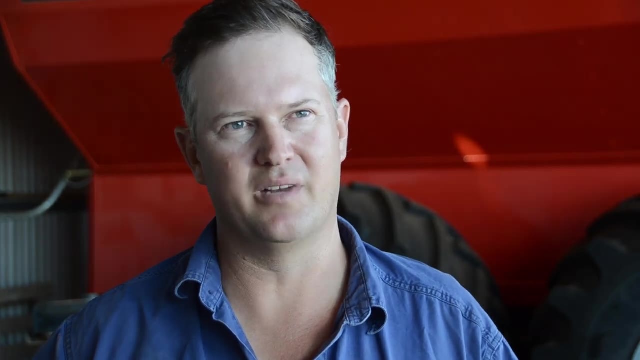 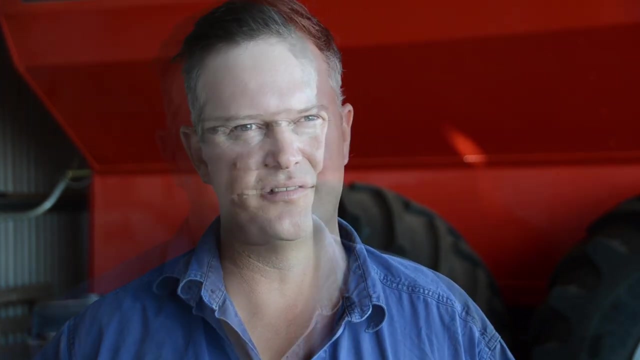 dynamic lifter down into that lower soil profile. that will promote plant growth, root growth and hopefully the moisture that's available down in that soil the plant can have readily available and hopefully increase yields. If we want to continue farming out here, we're going to have to grow crops more profitably.